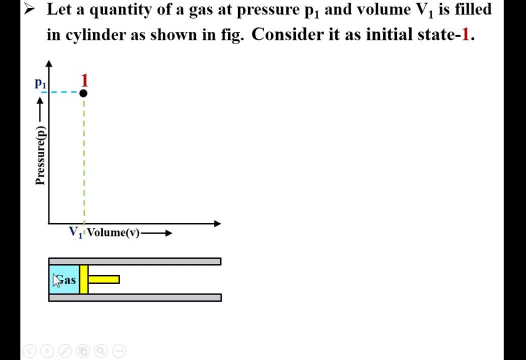 initial position of this gas. That means this gas having pressure P1 and volume V1.. Now this gas changes its state from state 1 to state 2.. So it has a pressure P2 and volume V2.. So here you can see the volume and pressure. both are changed and so that my final state 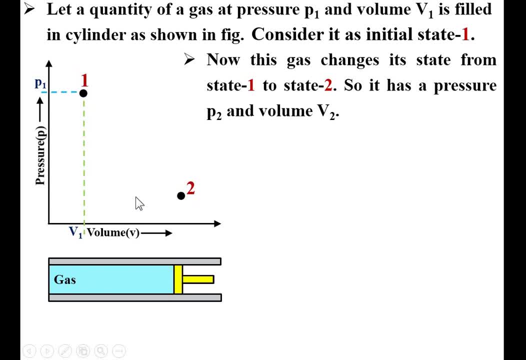 of the gas, it is over here, and corresponding pressure P2.. So I can write over here P2 and corresponding volume V2.. So now you can define the first terminology state. So it is condition of a system specified by Its properties. So any two independent property: either it can be the pressure and volume, or 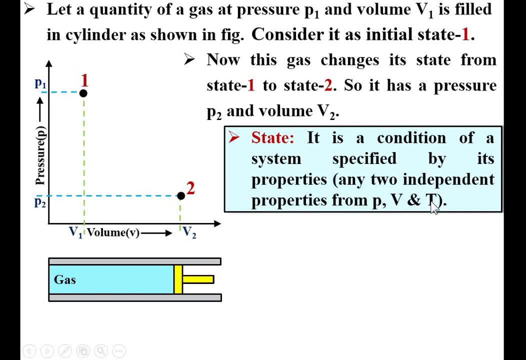 it can be volume and temperature, or it can be pressure and temperature. So here you can say: state 1: two independent property pressure P1 and volume V1.. Similarly for the state 2: two independent property, pressure and volume. Next terminology, that is the process, Any 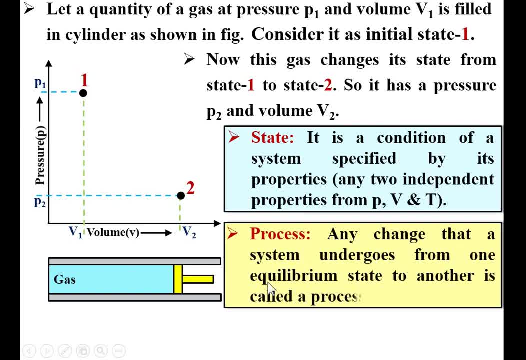 change That the system undergoes from one equilibrium state to another is called a process. So here it is equilibrium state one and this is the equilibrium state two. So any change from the equilibrium state one to equilibrium state to is known as process. here from this figure We can say: 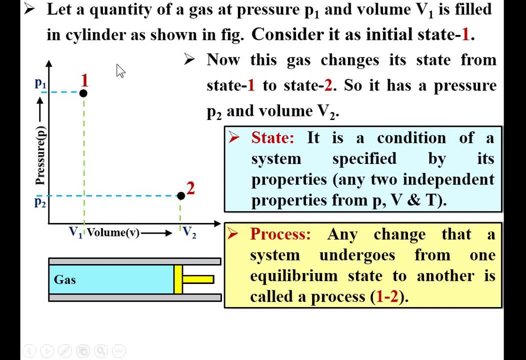 12 is the process. This is the process. Now, next terminology: path. The series of the states through which a system passes during the process is called path. So look at this word: series of the states through which a system passes. So here I am going to show the series of the states through which the system passes and 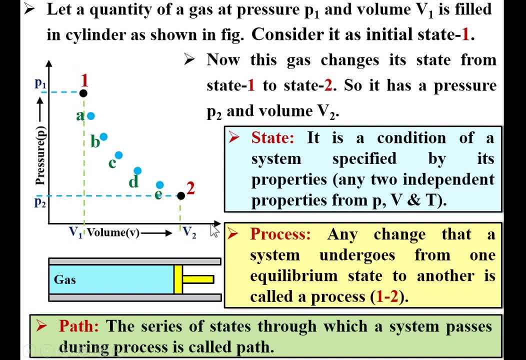 so that it will reach from the state 1 to state 2.. So here these are the intermediate states, and if I join it with the smooth curve then it will indicate the path. So I can write over here. this red color is the path of the process. 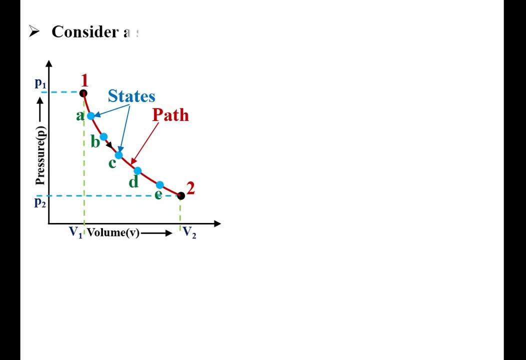 So this figure already we have discussed. Now consider a system undergoes by one more process to one. Now the same system undergoes by one more process to one. That means this gas changes its state from state 2 to state 1.. And so it has a pressure p1 and volume v1, as shown in figure. 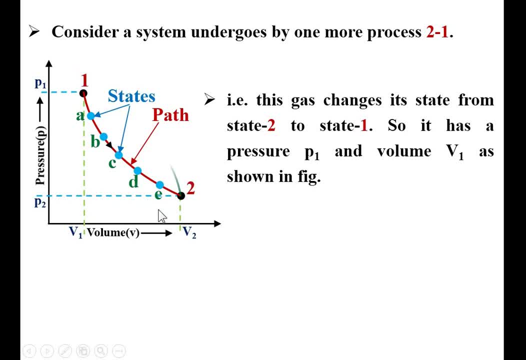 So I am going to show over here the process 2 to 1.. Here the path can be any one. So now I can define the last terminology. So I am going to show over here the process 2 to 1.. Here the path can be any one. 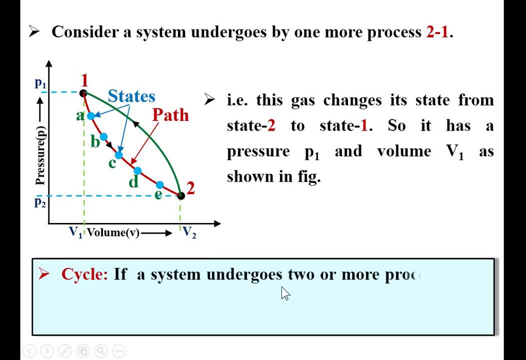 So now I can define the last terminology: If a system undergoes two or more processes. so here you can see one process 1, 2 and second process 2, 1.. So if a system undergoes two or more processes and returns to its initial state, 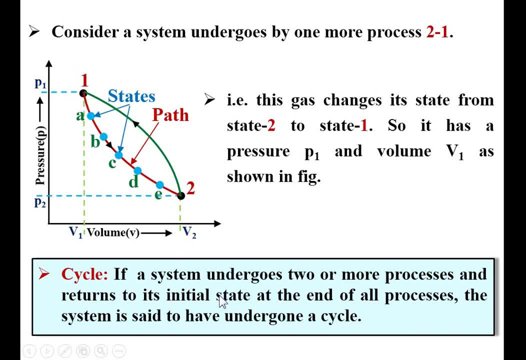 So here, this is the initial state. 1. So return to its initial state at the end of all processes over here. it is initial state. So this is the initial state. This is the one process and this is the second process. So the end of the second process. once again, it will come to its initial state. 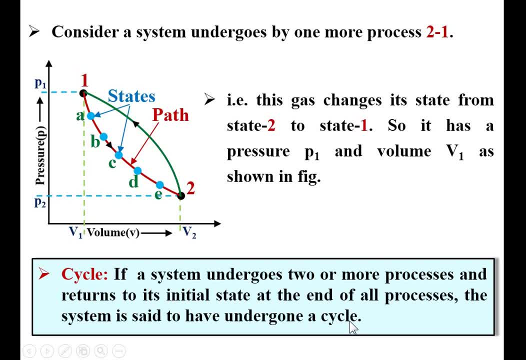 Then the system is said to have undergone a cycle. So we have discussed in this video the four important terminology. State, that is the 1 and 2.. Then process 1 to 2. And then path that you can see with the red color and with the green color. 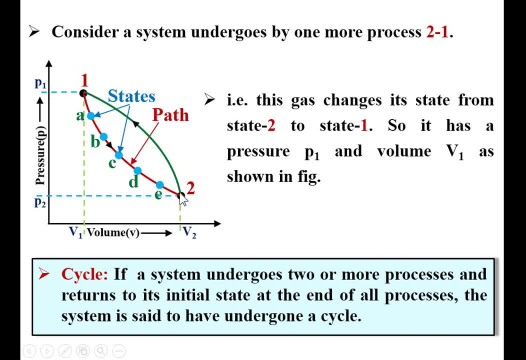 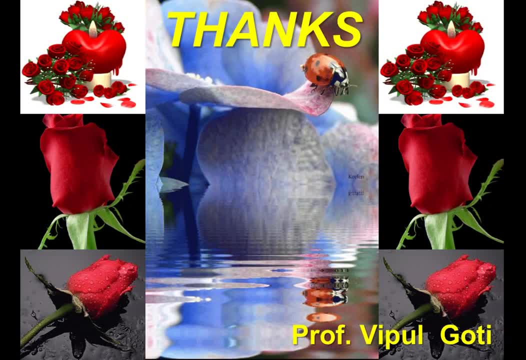 And fourth one is the cycle. So this whole 1 to 2 and 2 to 1 is known as the cycle. Thanks, my dear friends. Press like button to appreciate this video.